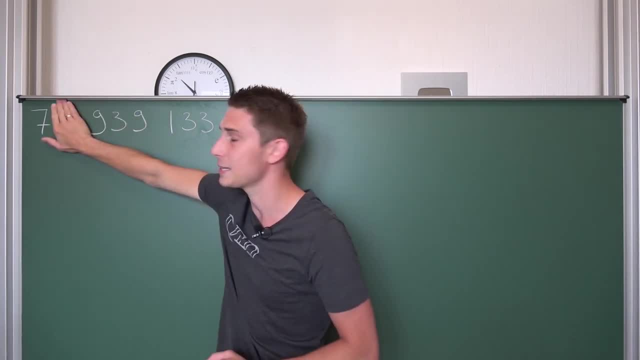 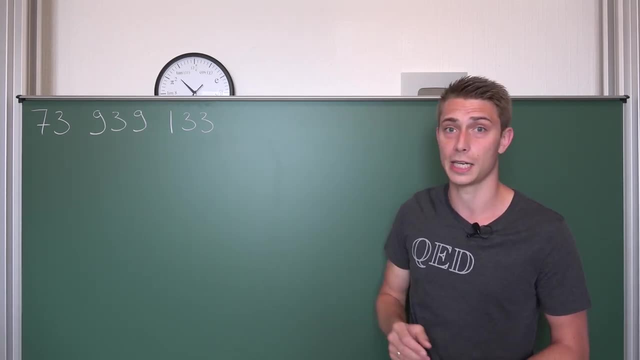 If we take another digit off, it's going to be a right truncatable prime, and so on up until the last digit. So that's extremely interesting, right? If you ask yourself if there are also left truncatable primes. so you take the left digit off and it's going to be a prime. Yes, those are out there. You can also generate a list of those. There are going to be more left truncatable than right truncatable primes. There are also truncatable primes which are basically from the left and the right truncatable up until the middle and so on. 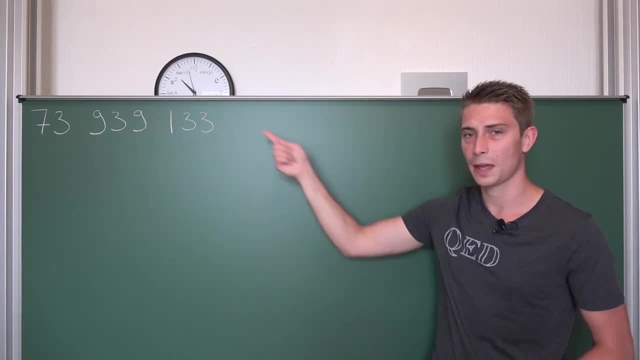 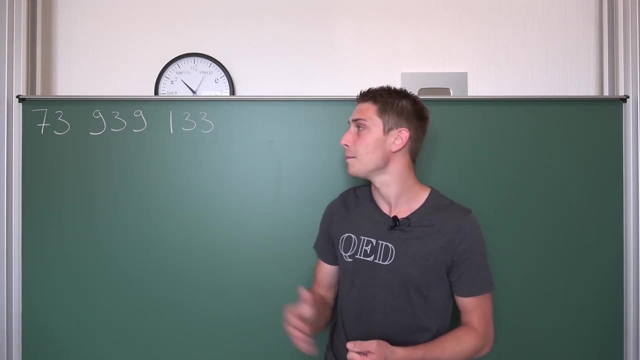 It's pretty interesting, But I choose the right truncatable primes Because that looks pretty sexy. if you ask me, Now we are going to dive into the mathematics behind right truncatable primes. Put some restrictions on the numbers that satisfy this very property. 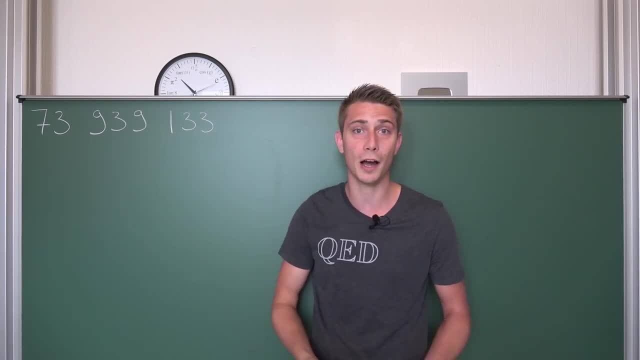 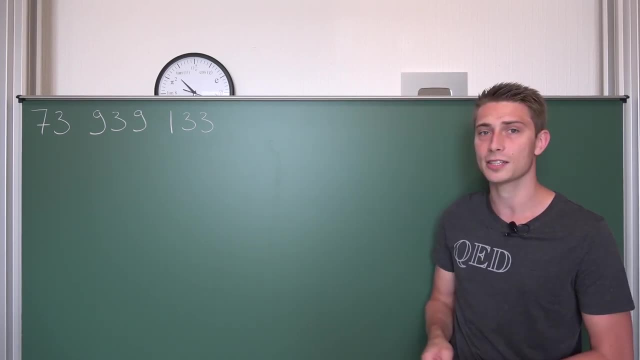 And in the next video we are going to implement everything into a Python algorithm. So yeah, we are going to dive right in. At first, I would like to play around with base 10 and digits. basically, I would like to take a look at the digit decomposition of some random arbitrary prime number with n digits. at first, 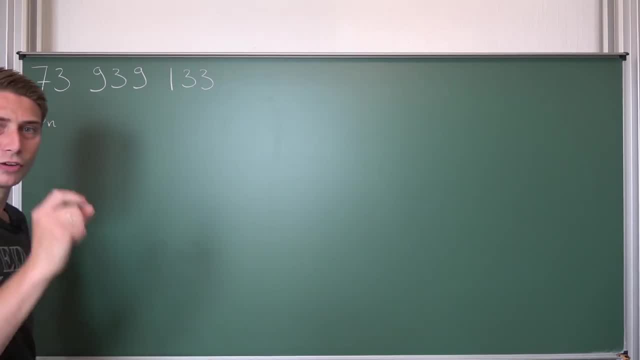 So we are going to have a prime number, We are going to call p with an index n. This n just basically states that we have n digits. Now, what's the digit decomposition? Well, it's just going to be the digit 1.. 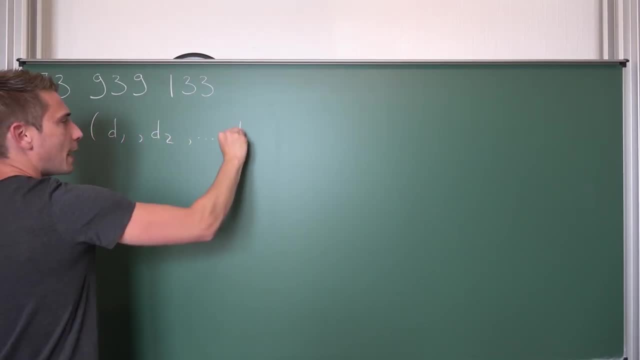 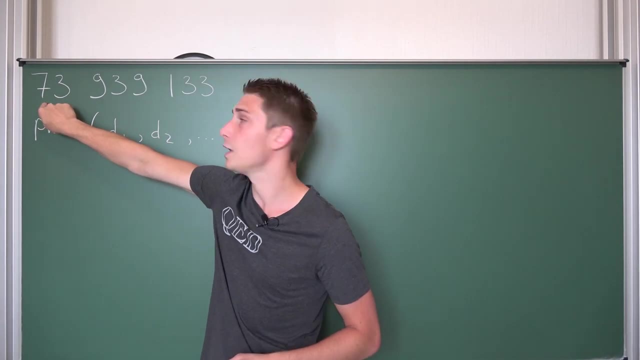 And then we have the digit 2.. It's just going to be a tuple up until the digit n. So think about it. Digit 1 is going to be, well, the first one here on the left, 7.. Digit 2 is going to be 3.. 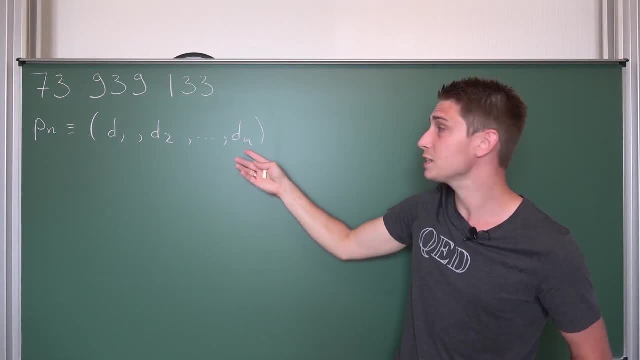 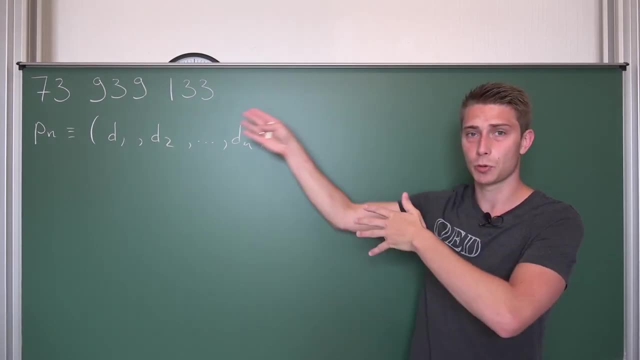 Up until the nth digit. we don't know yet how many there are going to be digits. The n is going to be 3 in our case, With this prime number up there. Okay, now we are going to induce the property of a right truncatable prime onto this digit decomposition. 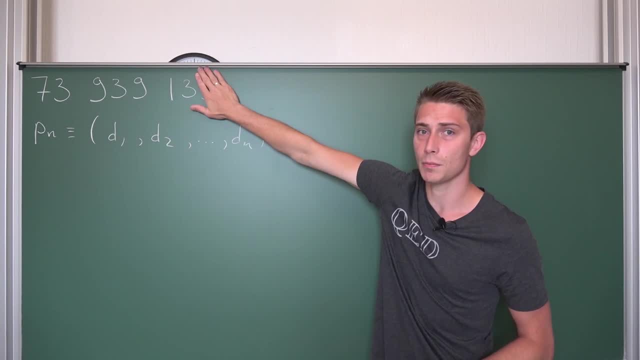 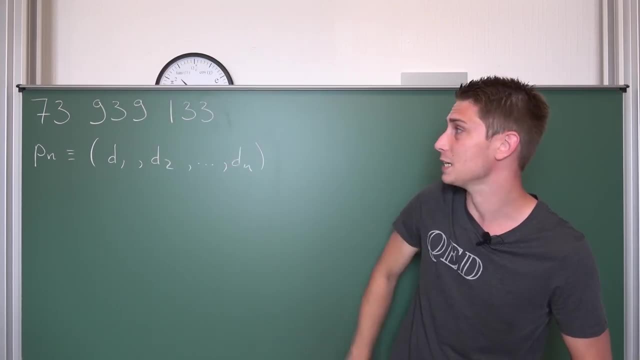 So what have we done? We took off the last digit, meaning prime number with n digits, turned into a prime number with n minus 1 digits, And the most important property is that all the other digits are going to be preserved up until the n minus 1th digit. 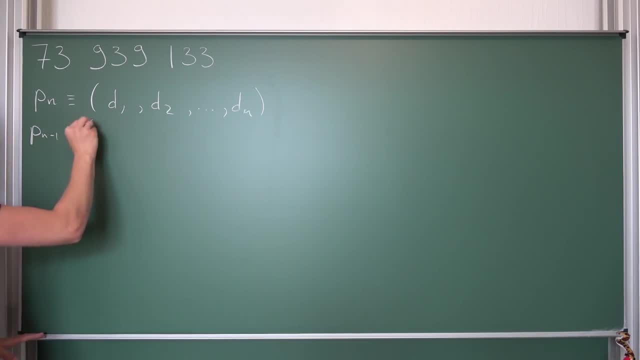 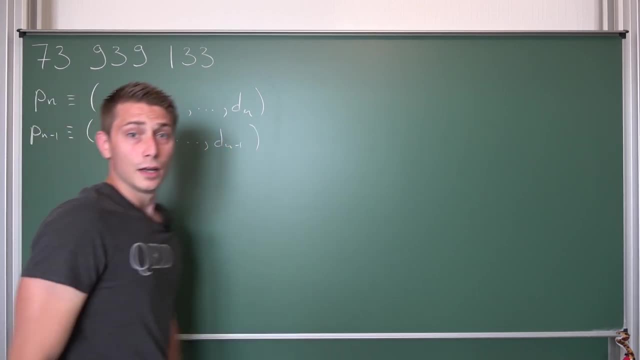 So, after taking a digit off, we are going to get ourselves a digit decomposition as follows: D1, D2, blah, blah, blah up until the n minus 1.. And so on. We are going to continue this process for it to be a right truncatable prime, up until the very last digit. 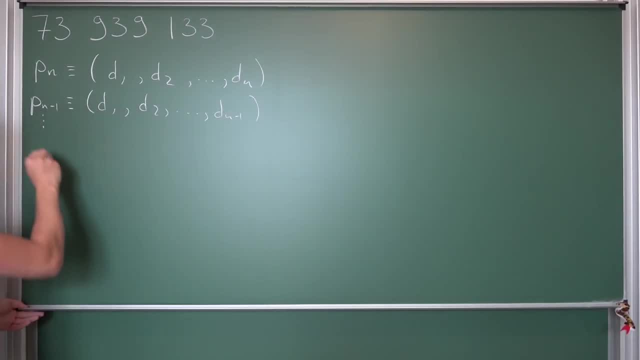 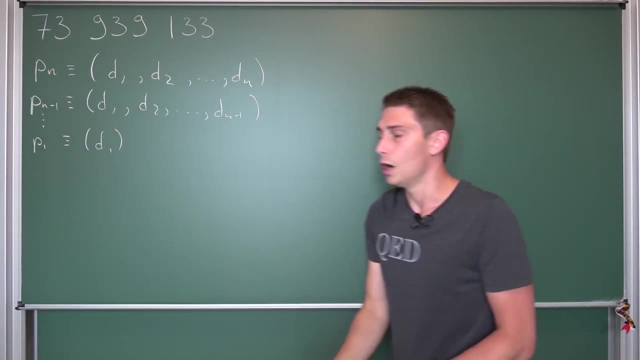 Meaning: after n minus 1 iterations, overall we are going to get to P1, which is just well, a prime number with a digit 1.. Okay, that was quite easy, but how does this help us? It really doesn't help us right now. 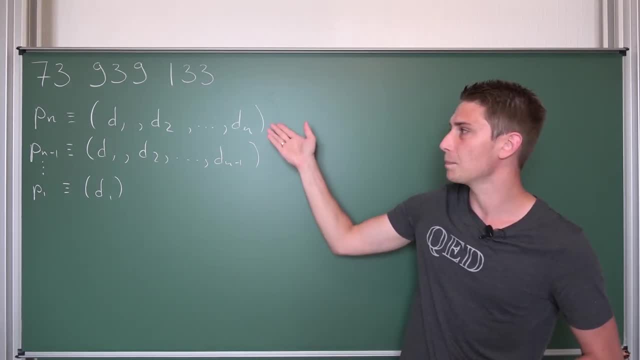 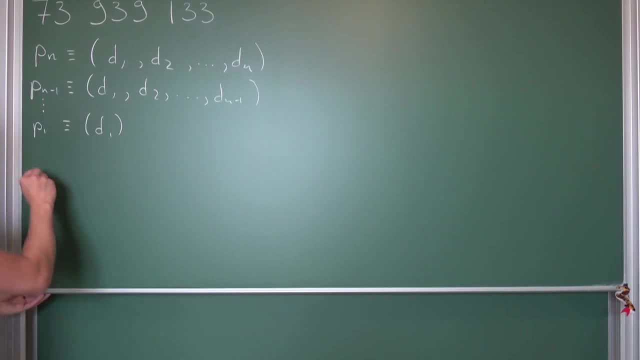 This is why we need to take a look at further emphasizing on what a digit decomposition actually is, And for this I would like to just take a look at my most favorite number. as a little example, Let us take a look at 135.. 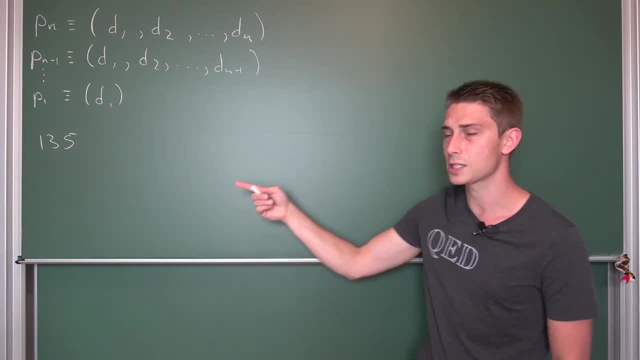 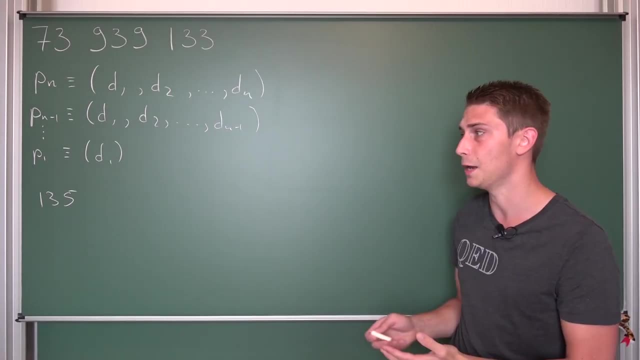 It's my most favorite number out there. And how can we decompose this into something in base 10?? Meaning we are going to decompose it into digits corresponding to powers of 10.. Well, at first let us write out what the digits actually are. 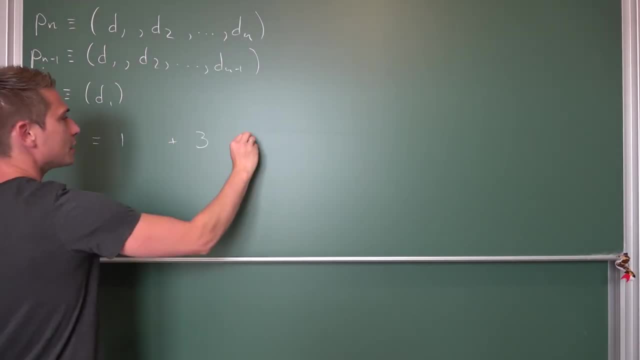 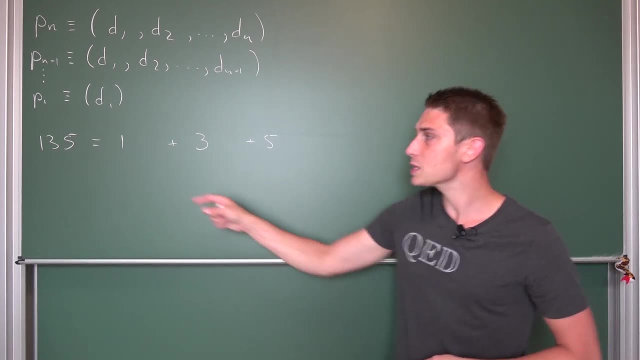 So our digits are 1.. Okay, We have 3 and the last digit is 5.. Okay, I hope you can see where this came from, But now they have to correspond to powers of 10.. Meaning, how is our 1, our digit 1, connected to what we have here? 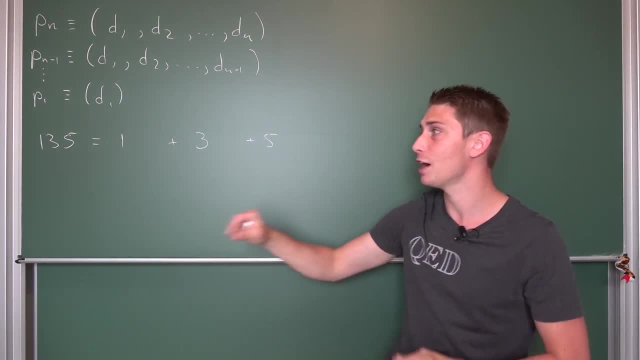 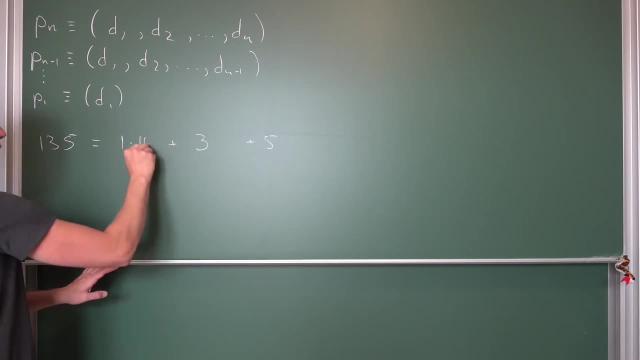 Okay, Think about the word 135.. Meaning our 1, digit 1, corresponds to number 100.. Our number 100 is nothing but well, 10 squared. I hope you can see where this came from. We have 100 plus and then we get 30 plus 5.. 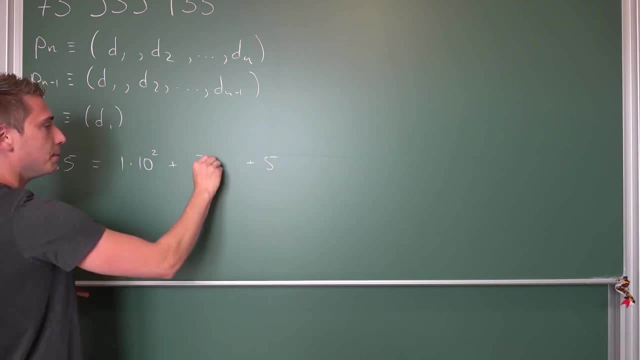 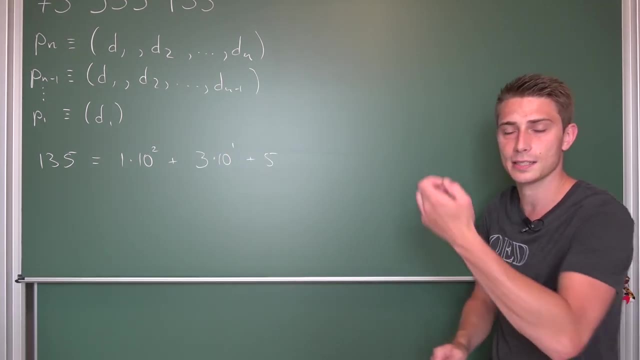 Okay, Our 3 corresponds to the number 30. Meaning the power of 10 is just 1.. Now our number 5 is just well, it's just 5. basically, times 1 and 1 is 10 to the 0th. 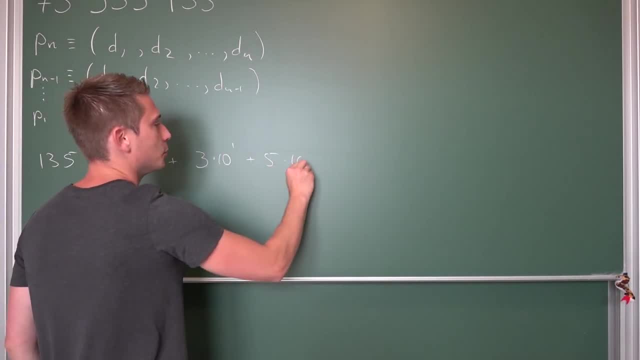 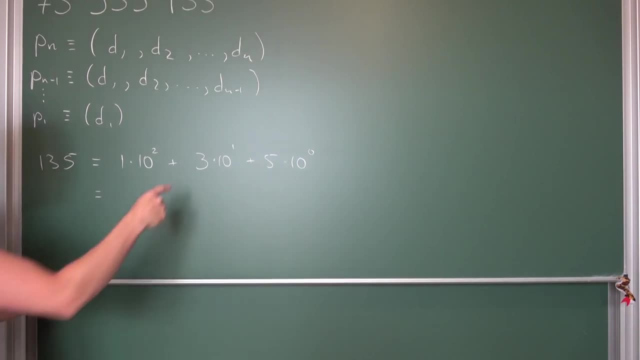 power. For the sake of notation, we are going to also put the 10 to the 0th power into here, Meaning overall, what are we getting exactly? I mean, if we were to put this into digit notation, we would get: okay, 1 is our d1.. 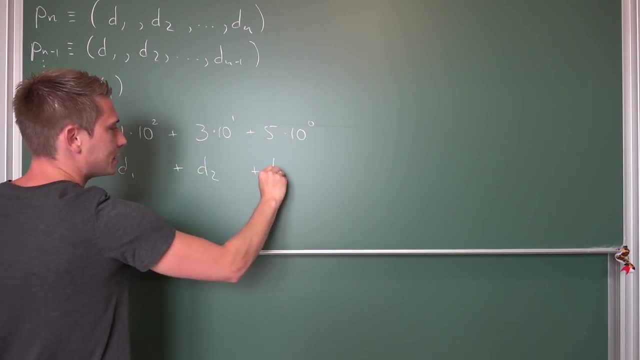 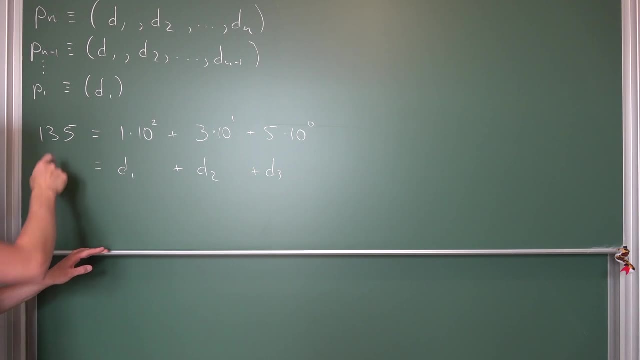 Then we have 3 being our d2. And then our d3 is going to be 5.. And take a look at the index. It ranges up until the number of digits. Okay, 3 is the number of total digits we have here in 135.. 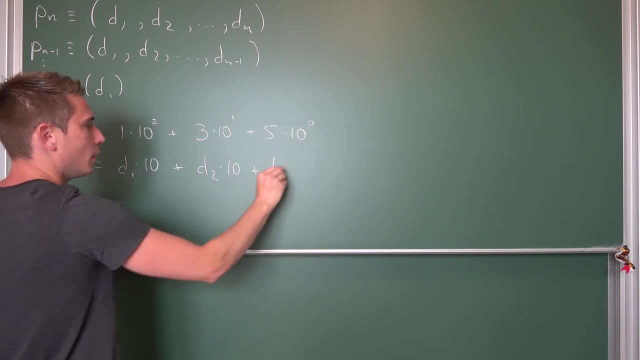 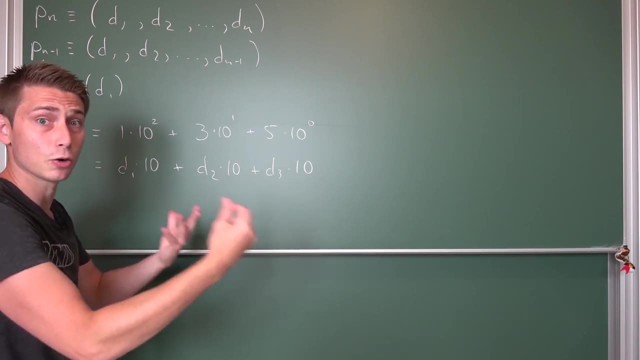 Now we also have powers of 10 in some way all the time, And now we need to see how those powers of 10 are connected to our total number of digits and the running index. we are going to sum up over: Okay, Now we have 10 squared. 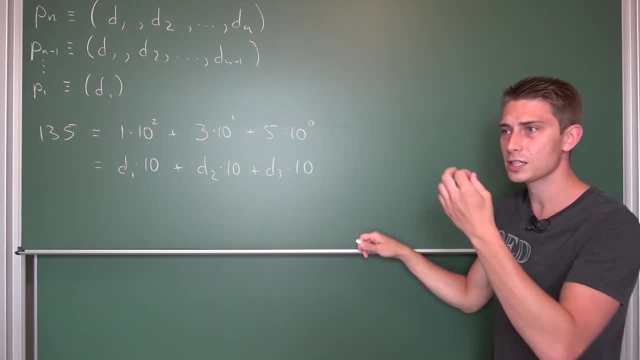 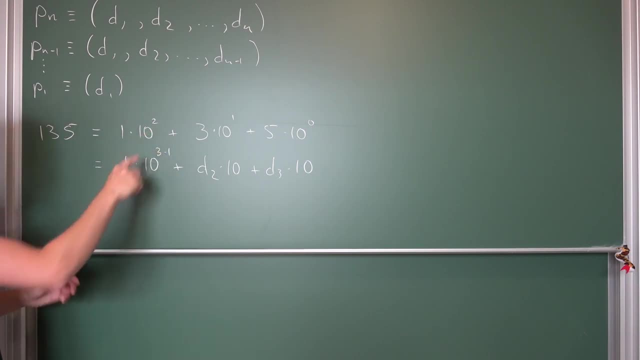 Now, how is 2 connected to 3?? Well, we are going to take the total number of digits. Total number of digits: 3. And we are going to subtract our running index from it. Okay, 3 minus 1 is going to give us 2.. 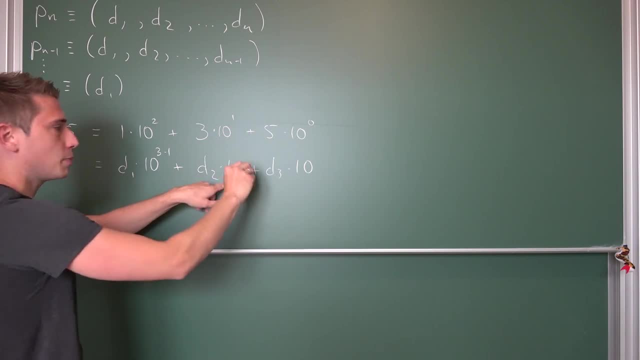 Does this pattern work out for the next one? I mean 10 to the first. power is just 3.. Total number of digits minus our running index, 2 that we are having here. Hey, it works out. Same should be here. 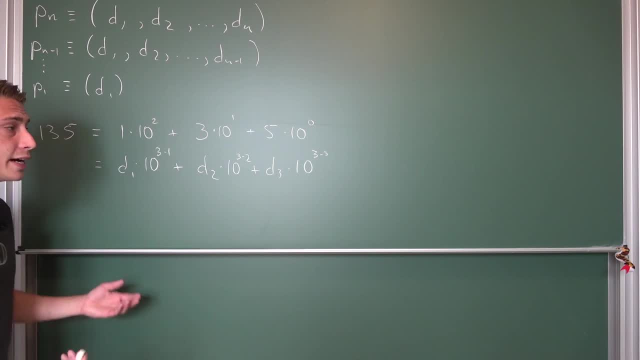 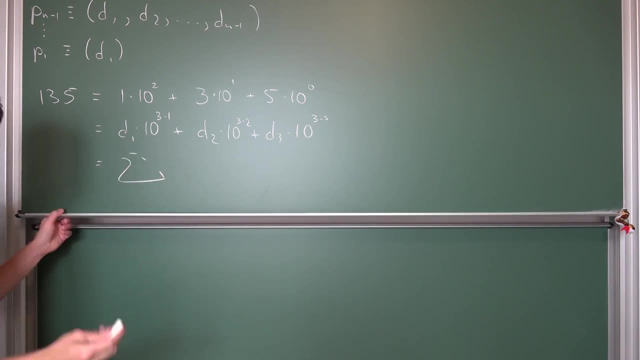 3 minus 3.. Total number of digits minus our running index: 3.. And thus we have found out a nice formula Meaning overall. if we were to put this into summation notation, we would get in some way a running index. 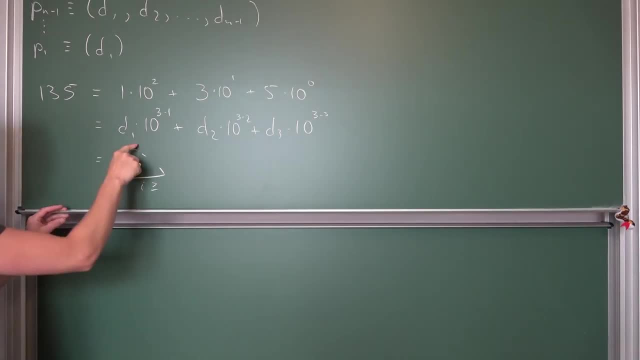 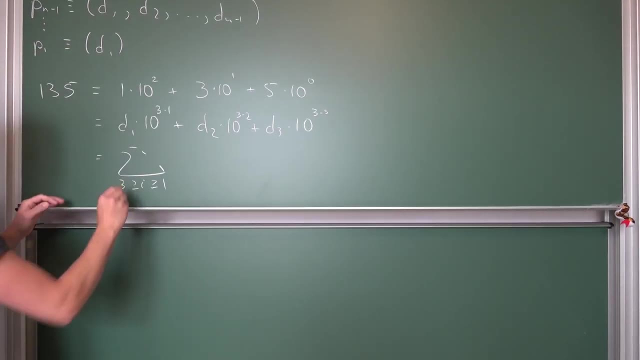 We are going to call it i, which is bounded between: okay, what's the lowest index? That is 1.. And what's the highest index? That would be n in some way, And our n is 3.. Okay, Now, how does it work for our digits? 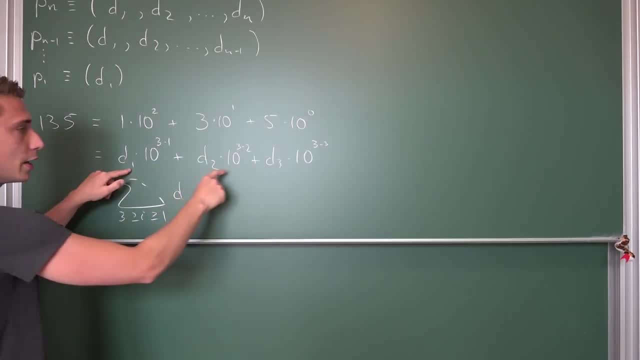 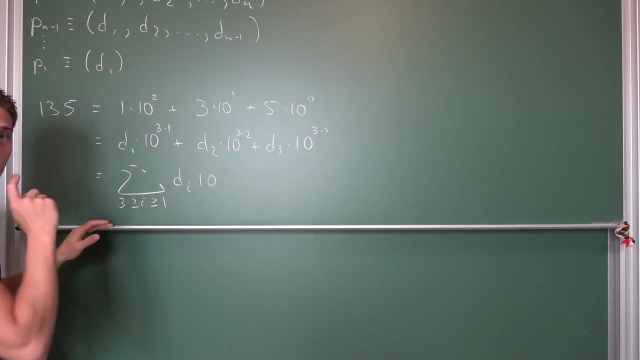 Our digits are just going to be raised by 1 all the time, So 1,, 2,, 3.. We are just going to count over the running index. Then we have 10 to the okay. what is constant up here in the power? 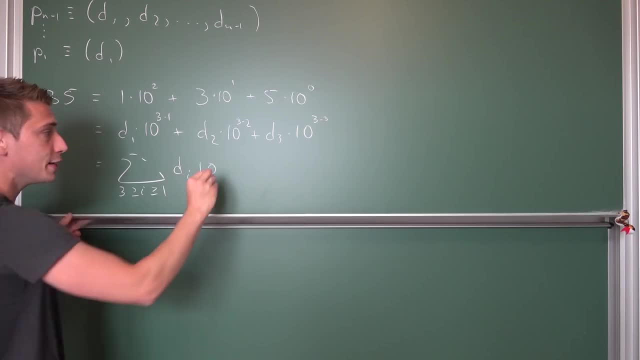 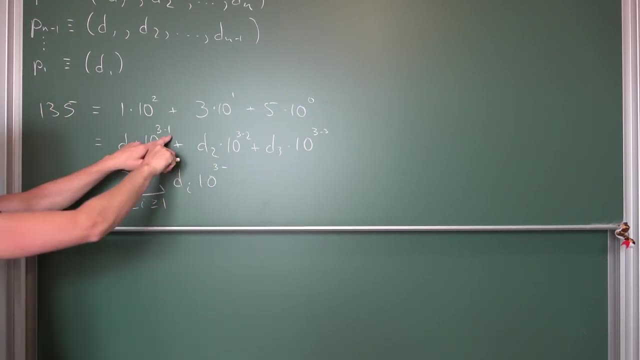 It's always the total number of digits, which is 3 in our case, Or For the most generalized version, it's going to be n, And other than that, we are going to subtract our running index from it, So i 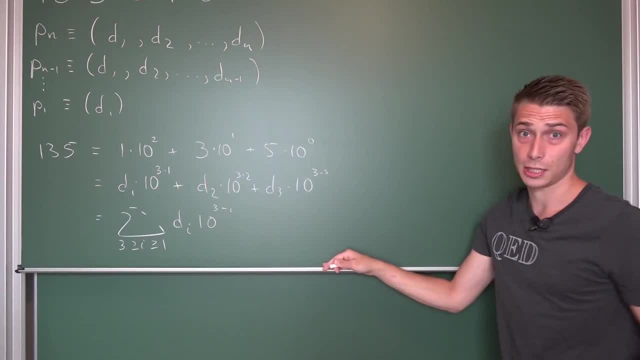 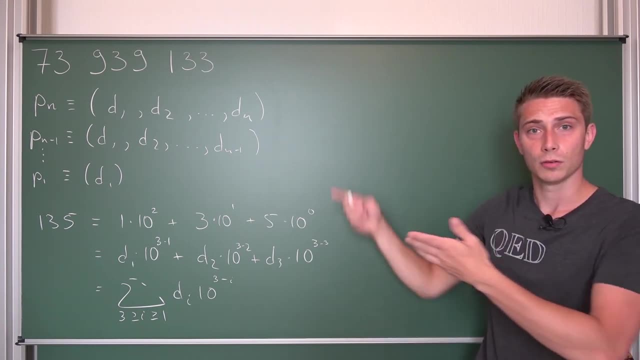 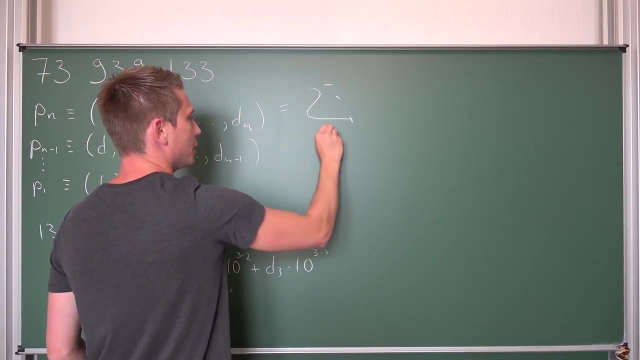 This is how we can decompose our 135 into a digit decomposition using powers of 10,, basically, and our digits. Now we are going to expand this knowledge upon those prime numbers that we have up here, Meaning overall what we have here. our Pn is going to be the summation where our running 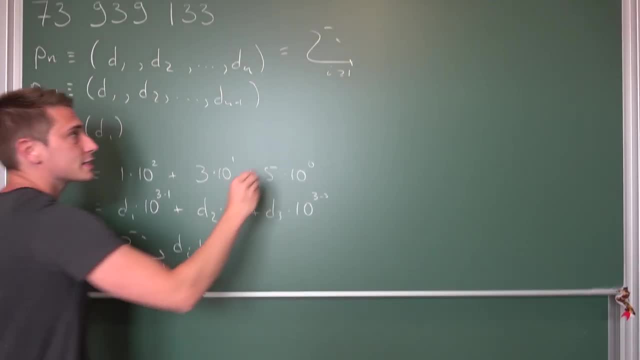 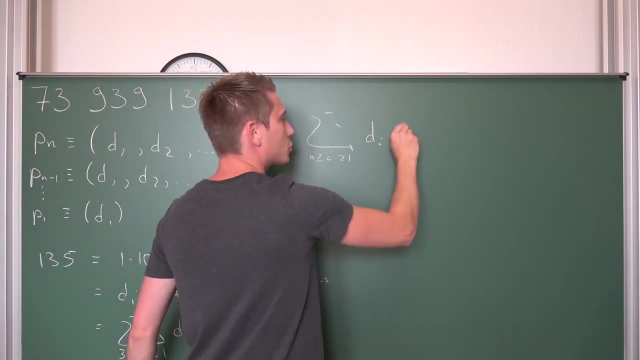 index. i goes from 1 to Well, now we have n instead of 3. And obviously we just have the same pattern. We are going to have our di's here And then we are going to multiply it with 10 to the 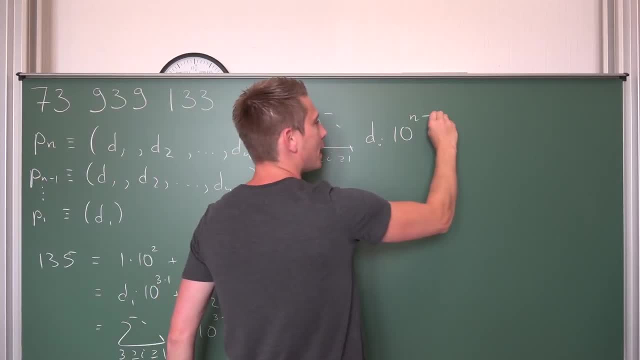 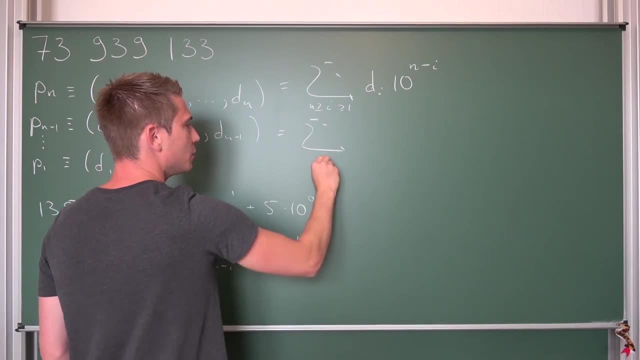 Okay, Our total number of digits is n, And then minus our i. Okay, What about our Pn-1?? Our Pn-1 is going to be well, just the same thing, just with n-1 instead of n. 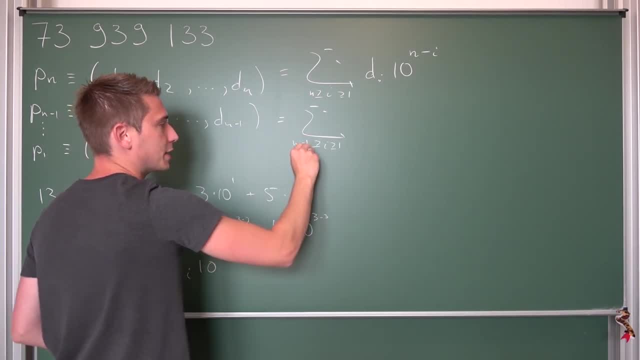 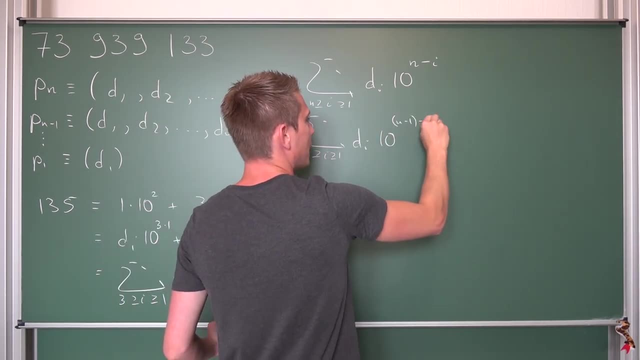 So our i is bounded between 1 and n-1 overall, And then we have di times 10 to the n-1 minus i power. Now we are going to write a bit more stuff out and we are going to see if we can find. 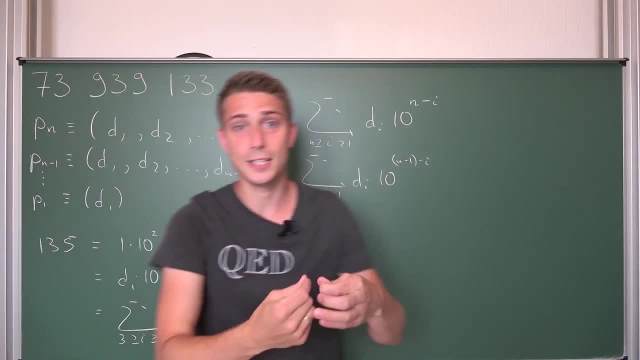 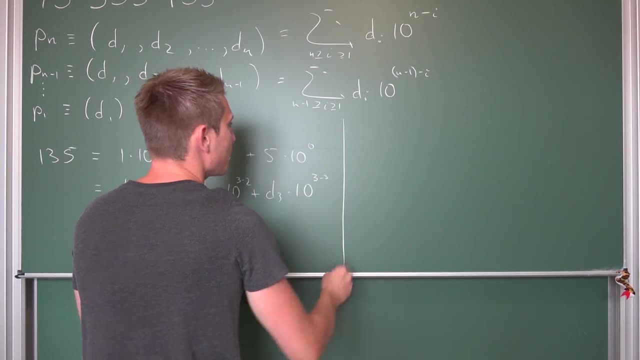 the connection between our prime number with n digits and our truncated prime numbers, Because this is a really important relationship that we need to take care of. I'm going to put this here. At first, let us write out what Pn actually was. 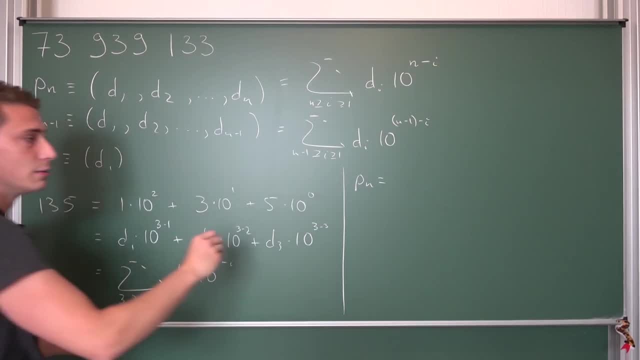 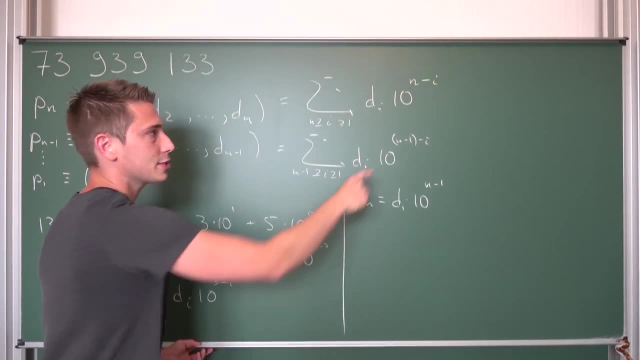 Pn was nothing but Okay. Now we are going to write everything out. This was the first digit: times t to the n-1 power. This is just the pattern that we are having here, Plus Then we have d2 times 10 to the n-2 power. 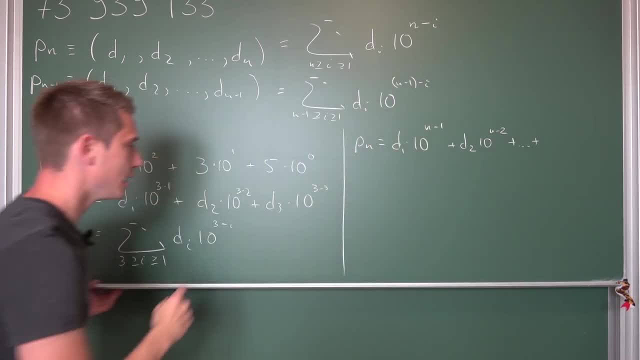 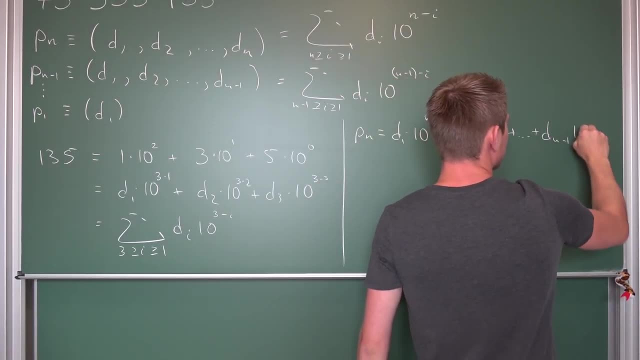 Plus Blah, blah, blah, Up until Okay. Then we have dn-1 times 2 to the first power- This is always going to happen- dn-1 times 10 to the first power, And the last digit that we are going to have is just dn. 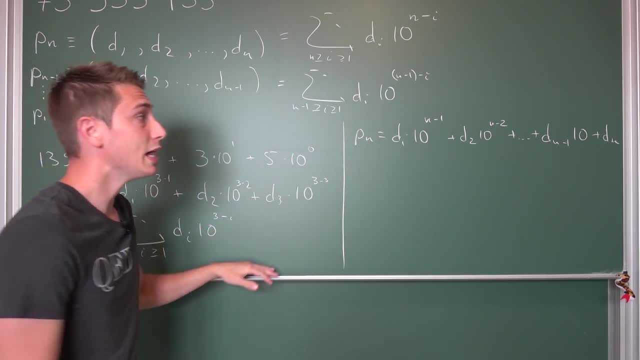 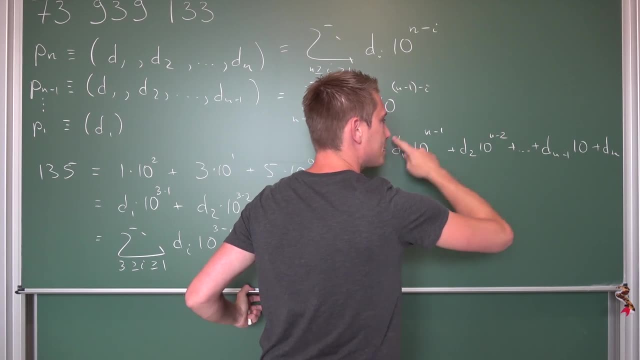 Okay, How can we continue from this point onwards? Well, It's not really obvious, but this is how I continued. You see that we have 10 as a common factor up until this nearly last term. Okay, One term before the last term. 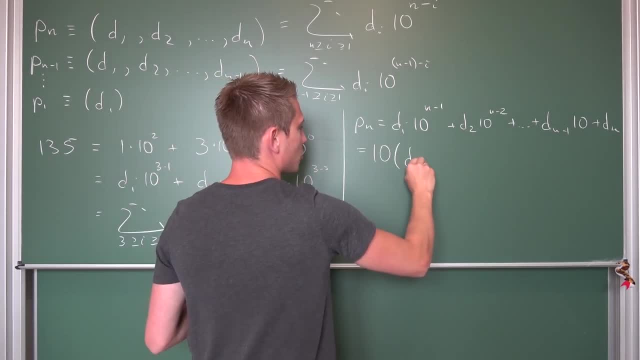 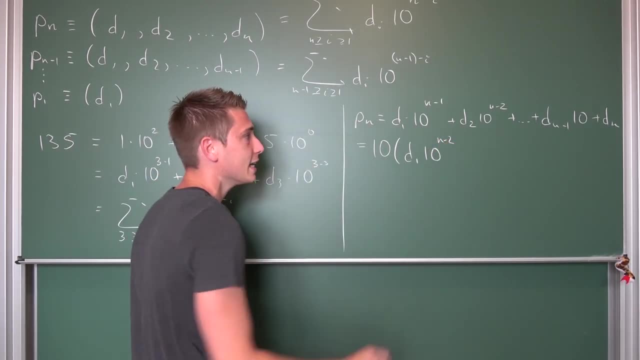 Meaning we are going to factor out the 10 right here, Leaving us with d1 times. Okay, Then we are going to get 10 to the n-2 power. Okay, We factored out the 10.. And then plus d2.. 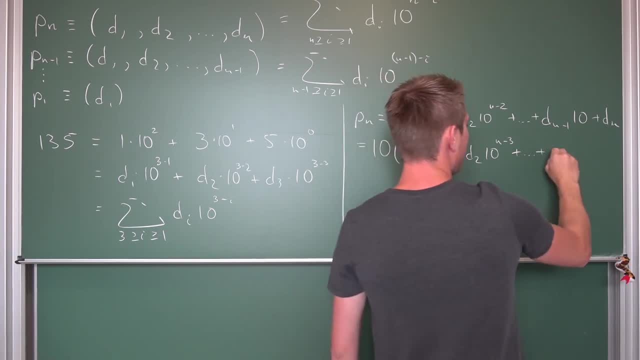 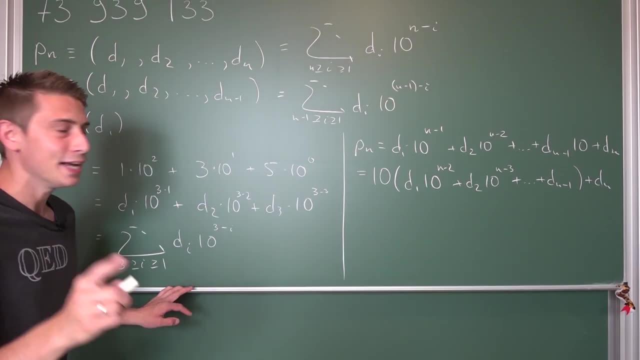 10 to the n-3 power Plus blah, blah, blah Up until, Okay, dn-1 plus dn. But how is this going to help exactly? Well, Now I want you guys to take a look at this right here, And we are going to write it out a tiny little bit. 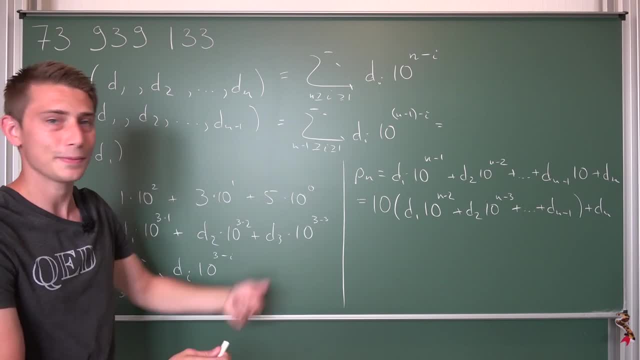 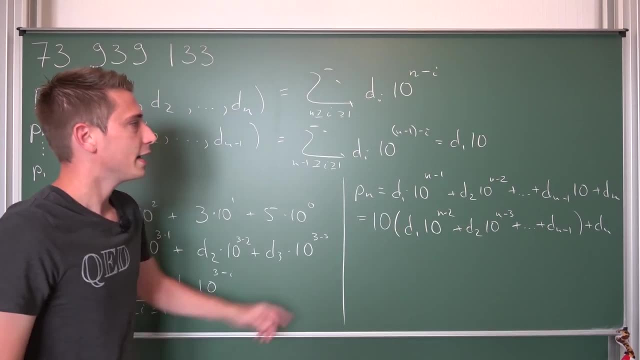 How about we write out the first and the second, And maybe up until the last term? So we are going to get d1 times Okay, 10 to the n-1 minus 1.. This is n-2. Aha. 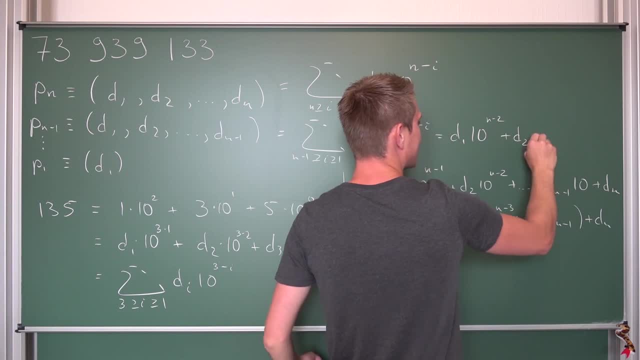 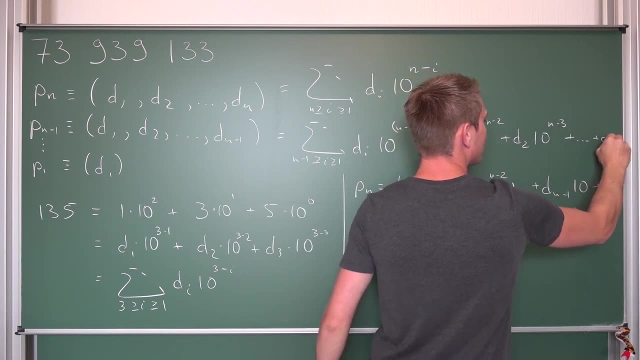 This is cool, Right, Plus, And then we are going to get d2 times 10 to the n-1, minus 2 is going to give us n-3.. Plus, Blah, blah, blah Up until d, And the last index is n-1.. 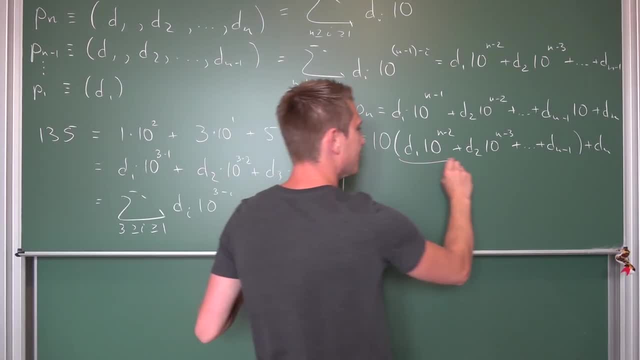 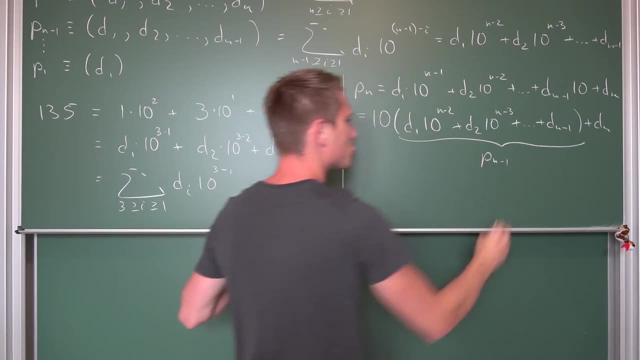 This is cool, Right, What we have here is exactly our pn-1.. Okay, I had to look for it, So we have pn-1 here, Meaning overall Pn. The nth prime number in some way can be expressed as: 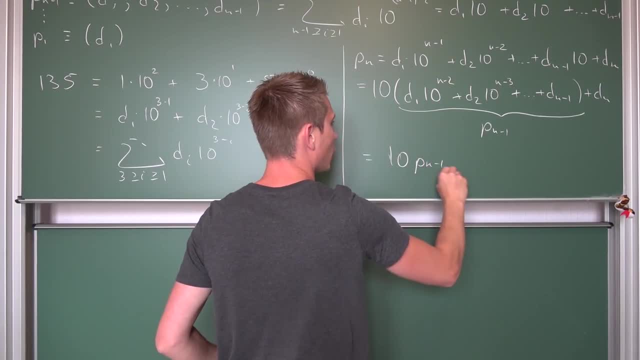 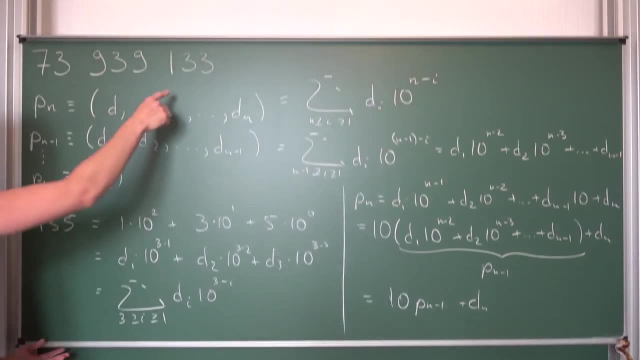 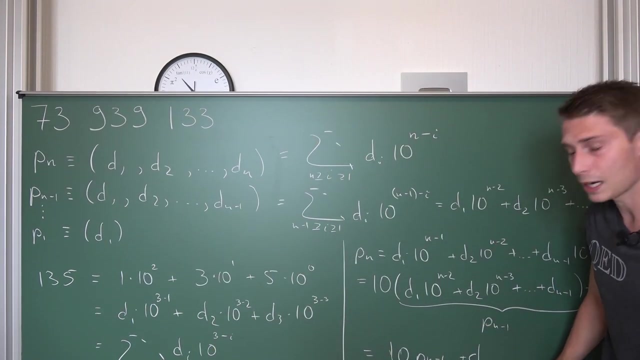 10 times pn-1 plus the last digit, dn, And this is going to help us a lot Finding out what our digits, that we can append basically to the very first digit, are going to be. Now We are going to write it out yet again. 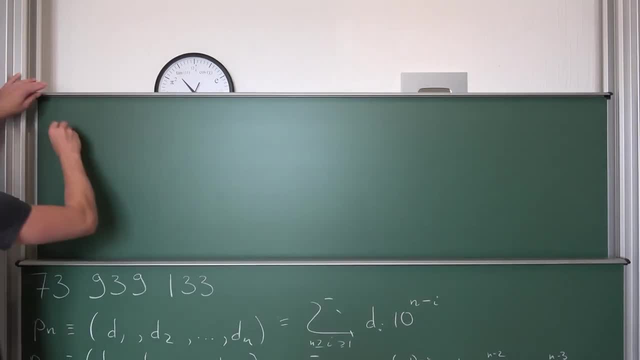 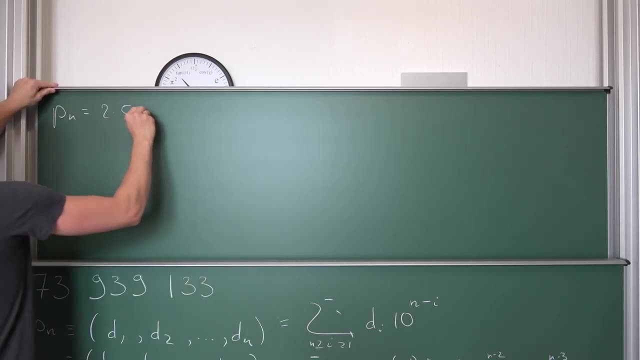 And we are going to take a look at some modulo calculations. So we have that pn is nothing. but What is 10 exactly in this prime factorization? It's 2 times 5.. Times pn-1.. Times pn-1.. 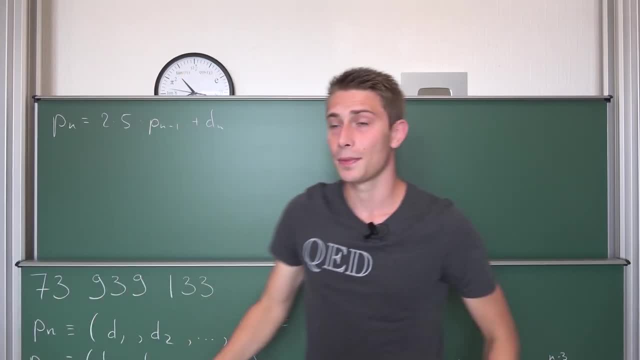 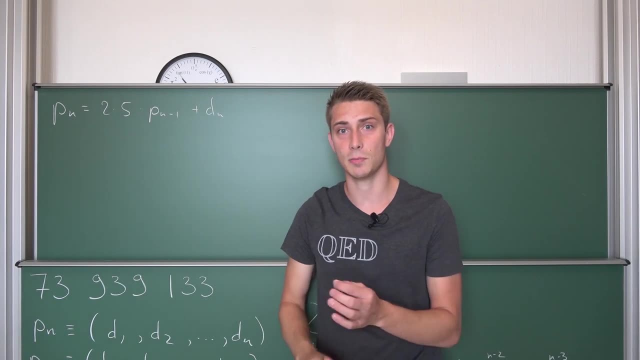 Plus dn. And now Here is one key fact that comes in with prime numbers: Prime numbers, Pn, Are only divisible by 1 and themselves Meaning. If, for example, Our dn Were to were 2. Then we could factor out the number 2 right here. 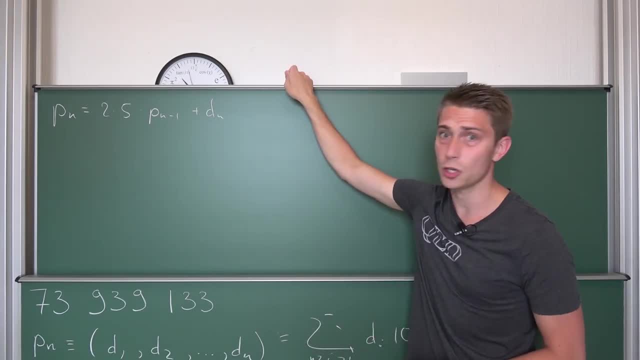 And thus pn would be divisible by 2.. Doesn't work out. What about dn being equal to 4?? Well, 4 is nothing but 2 times 2.. We could factor out the 2 yet again, And thus pn would be divisible by 2.. 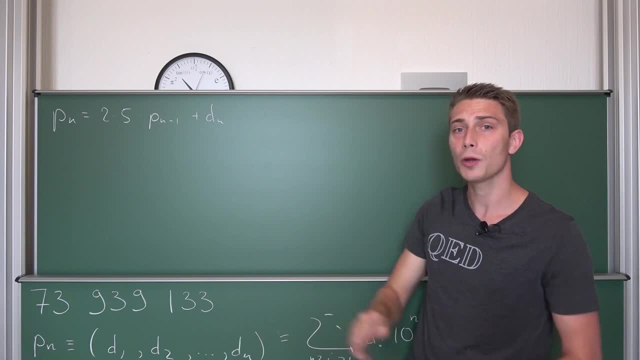 What about Dn being equal to 4.. Well, 4 is nothing but 2 times 2.. We could factor out the 2 yet again, And thus pn would be divisible by 2.. What about Dn being equal to 4.? 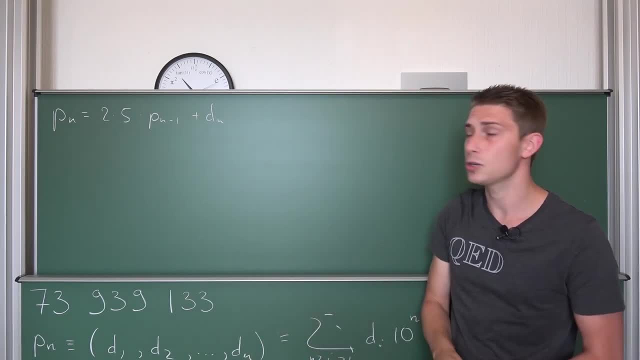 Well then, Our pn is divisible by 2. And 5., Which wouldn't work out Meaning overall, If we were to take a look At modulo calculations, Our dn right here Must not be congruent To 0.. 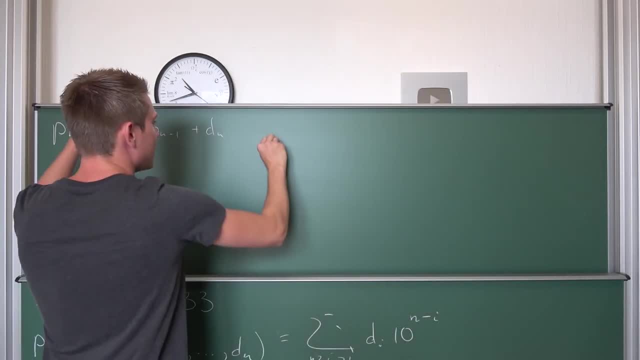 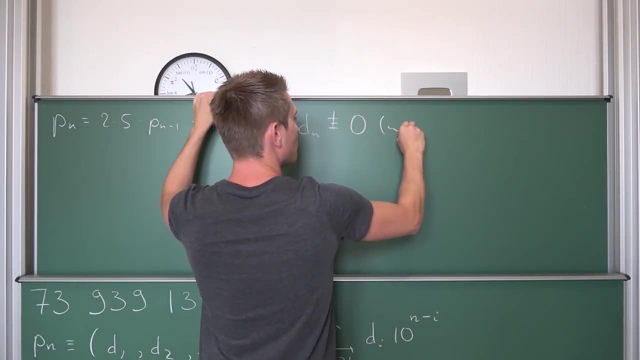 Modulo 2.. Or It must not be congruent To 0. Modulo 5.. What this means Is That Our dn Must not be congruent To 0. Modulo 2.. Or 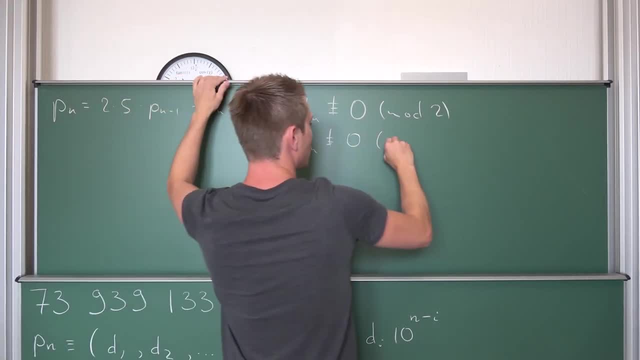 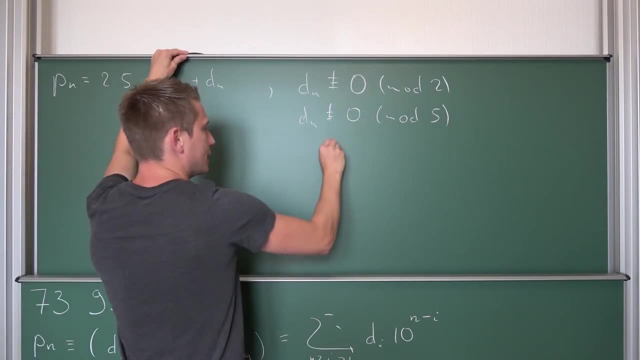 It must not be congruent To 0. Modulo 5.. What this means Is That Dn In general Is That we can restrict Our dn Right here. Dn Must Be element. 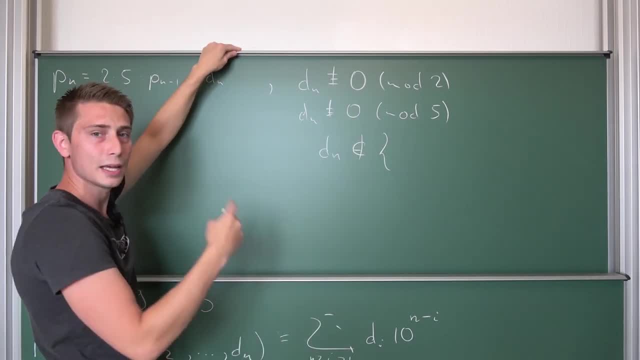 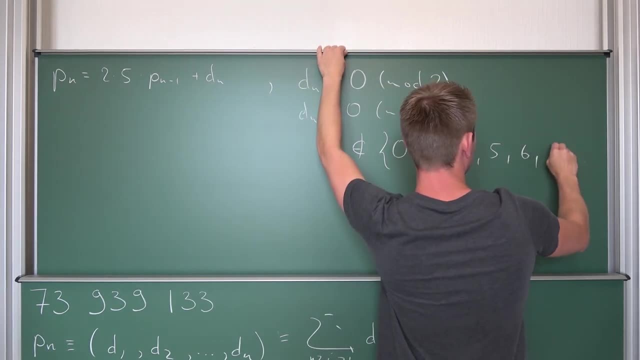 So Or Must not be element. Let's put it like this, If we were to take a look At the modulo: Must not be element Of 0. And then we have 2., 4., 5.. 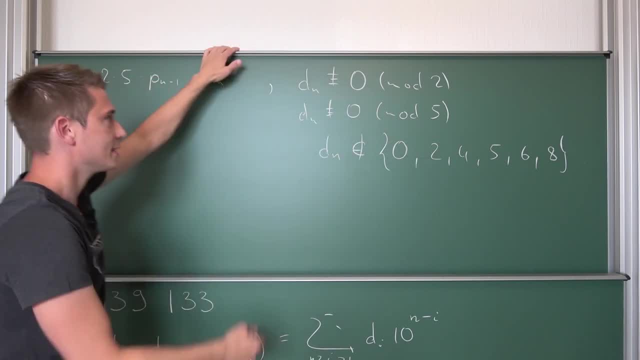 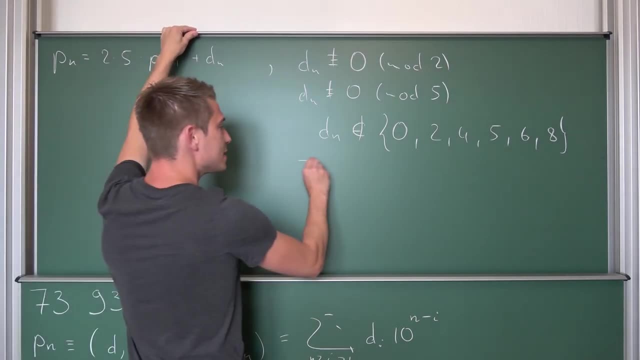 6. And 8.. Ok, If it is Any of those elements, It's not going to work out, Because pn Would be divisible By some number, For example. This Overall Means That our dn Must be element. 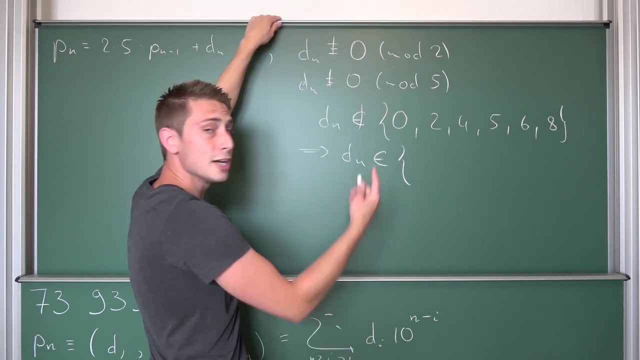 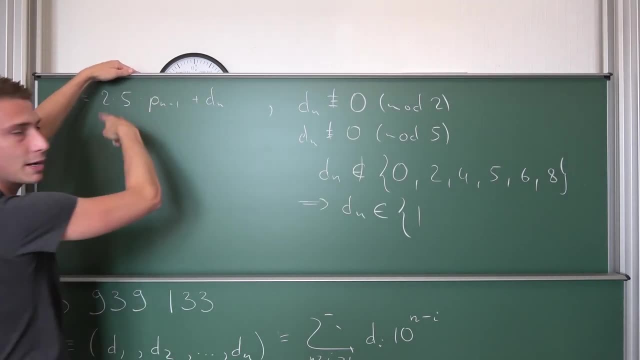 Of all the numbers, All the other digits Not in the set Right here. So What's not in the set, Ok, Dn Could possibly be 1.. This would work out If it were 1. We don't have any other factor. 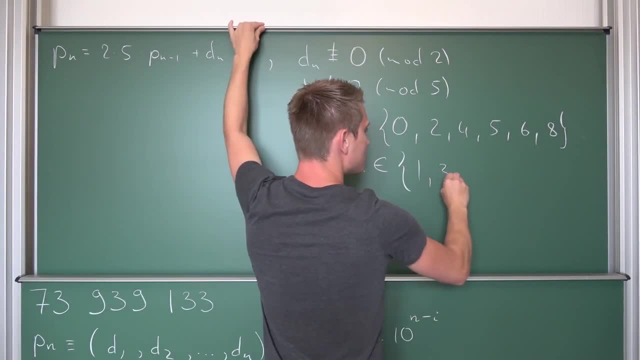 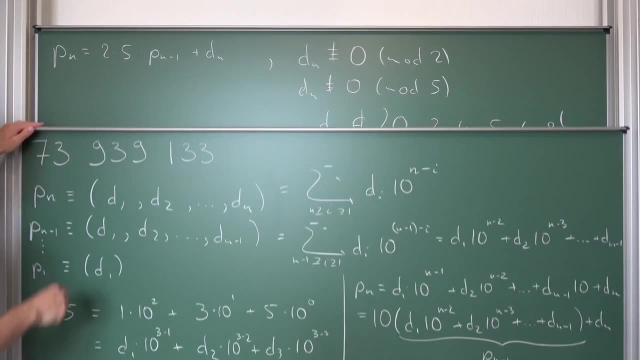 Which can be shared by Those two terms. Ok, It could be 1.. It could be: Ok, 3 is missing. It could be 7.. Or It could be 9.. And If you take a look, 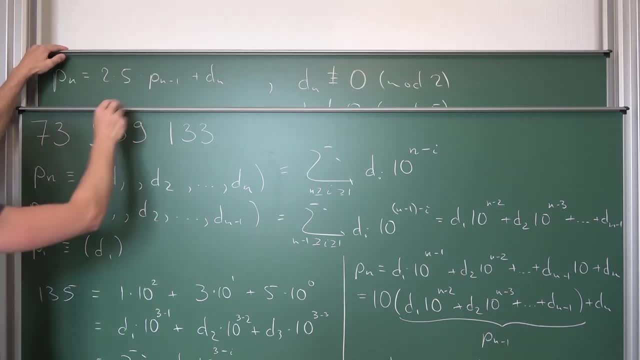 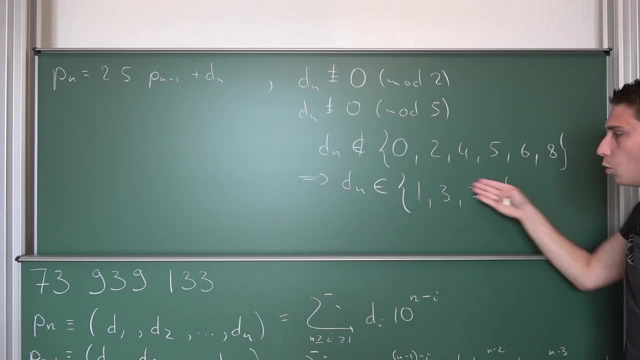 Those are exactly The digits We have here: 1., 3., 9. And also 7.. At the beginning The first digit Is a bit of an odd one Out, Because It doesn't really need to satisfy. 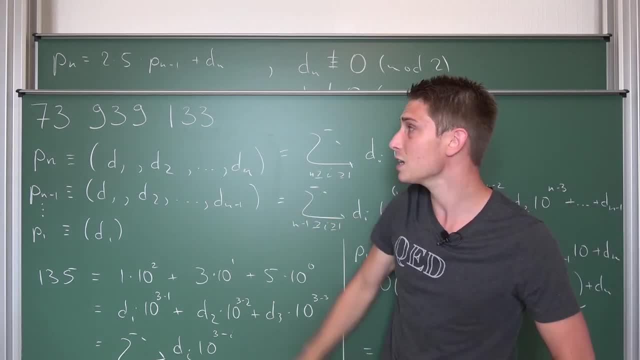 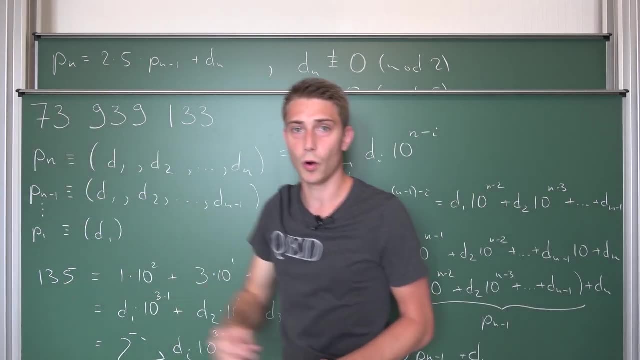 What we have here. Just because If you were to write A python script, For example, Or just take a look At this digit decomposition, It could be any Or prime number That you can find, Because the last digit 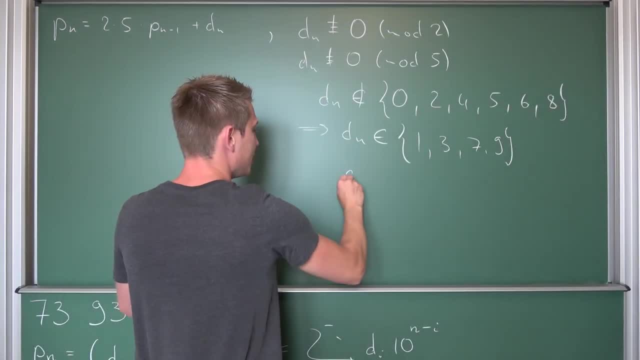 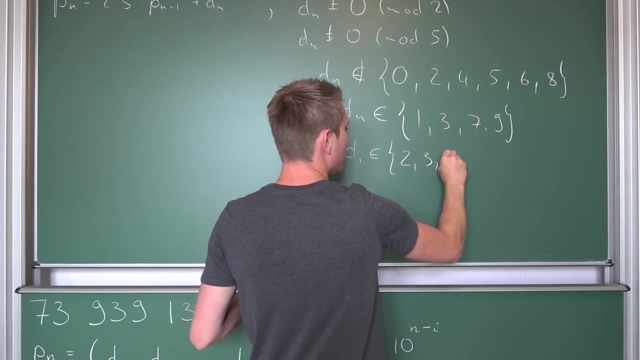 Must Only be A prime number Meaning overall. Our first digit Must be element Of all the Single digit Prime numbers That you can find. So, for example, 2., 3., 5. And 7.. 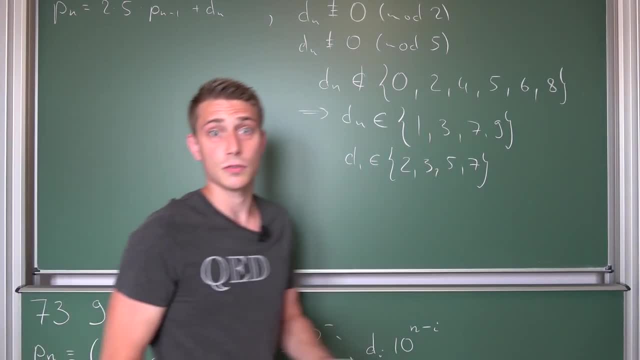 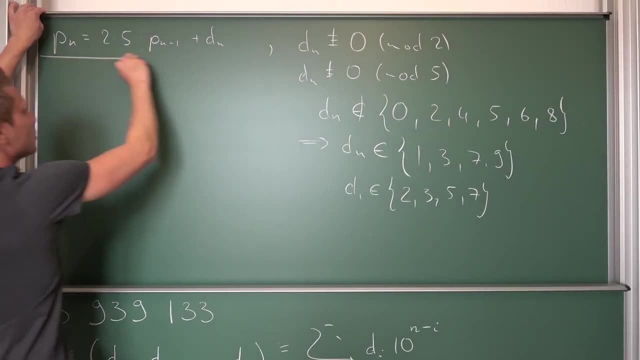 This is what they could Possibly be, And this is all the information That we need To create ourselves A list Of All the right truncatable Primes That there are. So Meaning, If you were to implement this. 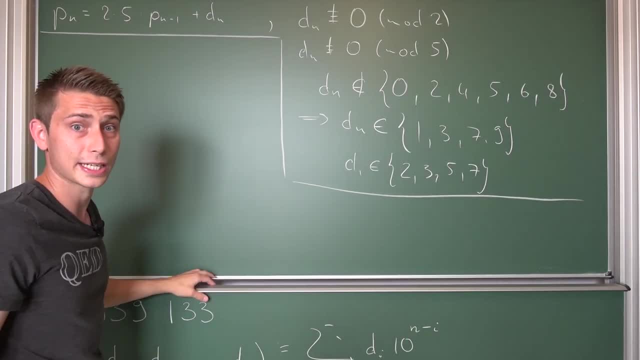 Into a python script, And this is the most efficient one I could come up with. It gives you the list Of all the prime numbers Which are right truncatable. Now, How does this work? So at first, We are going to start off. 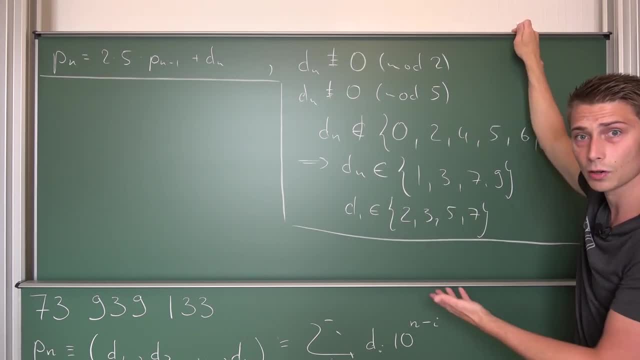 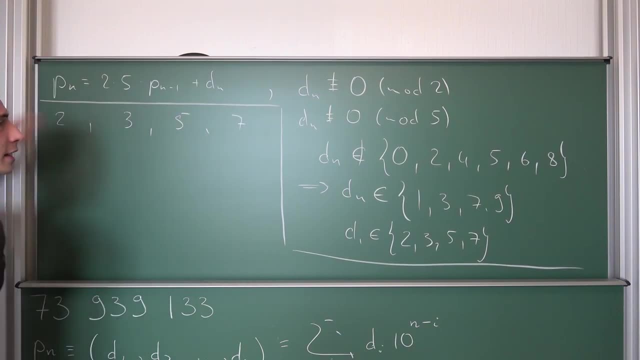 With D1. We are going to Get ourselves A list Of all the D1's, So the first digits, Which is a list of 2., 3., 5. And 7. And what we are going to do. 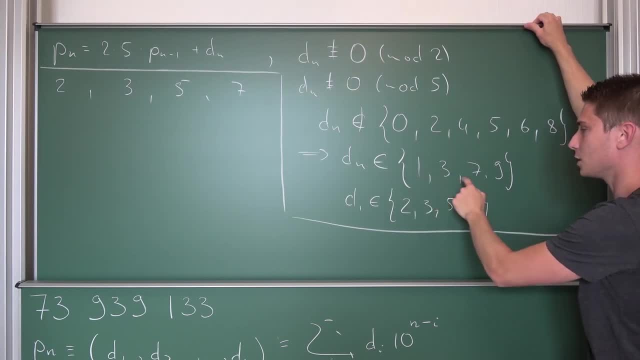 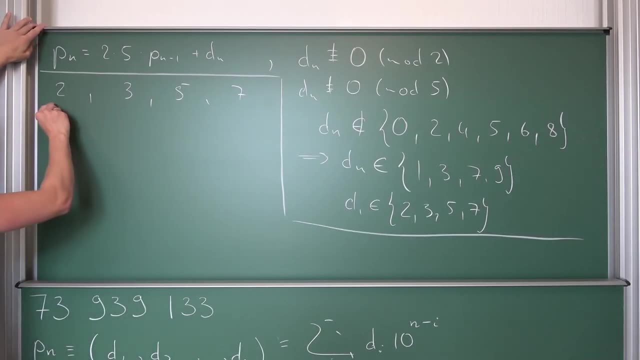 Is, we are going to create Ourselves Another list Which includes Those other digits, Those Dn's, Which we are going to append To this string. Basically, Now, What this means Is That we have: 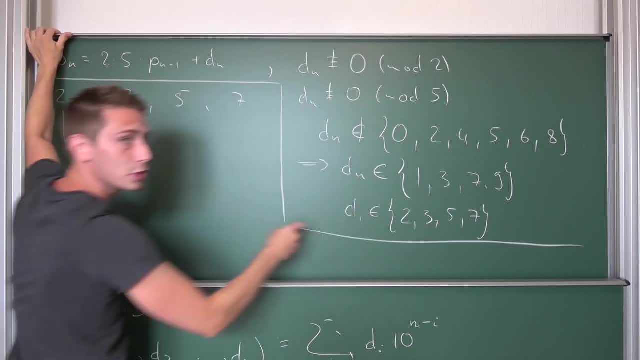 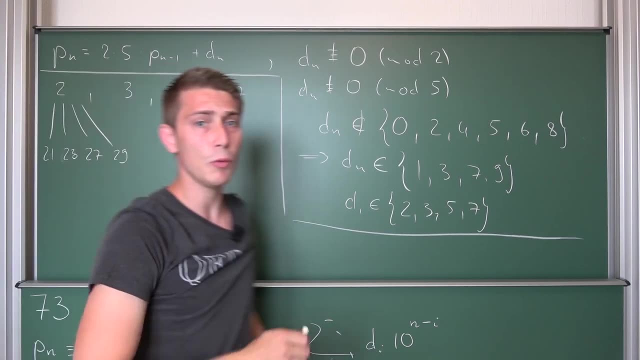 4 possibilities For number 2. We can append 1., 3., 7. Or 9. To it. So we have 21., We have 23., We have 27. And we have 29.. And now, 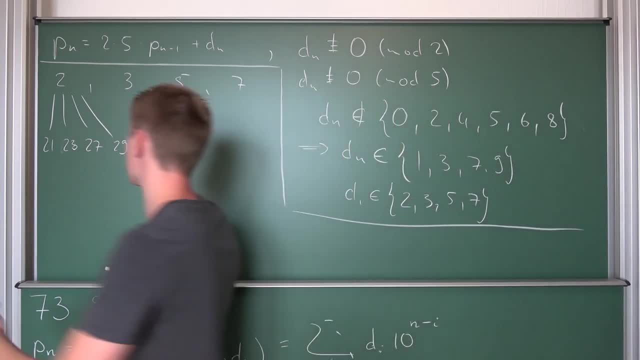 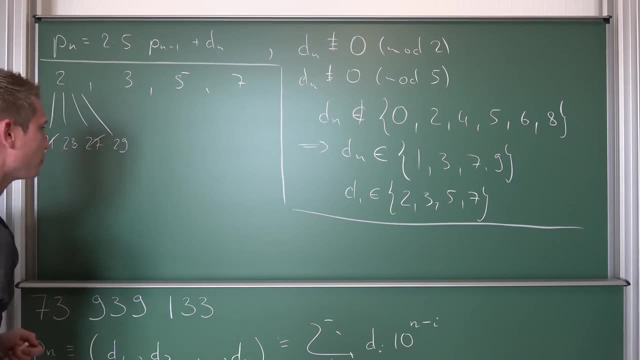 We are going to Let an algorithm run Which checks If those numbers Are prime, Because, Well, We need them to be prime numbers. So 21 is not prime, 27 is not prime, So 23 and 29.. 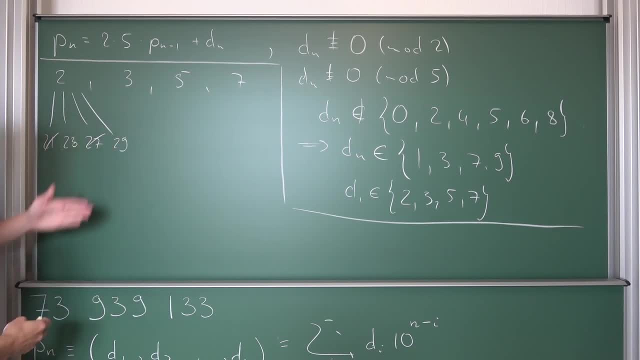 Are right- truncatable primes- Just because We can take the last digit off And we are still going To get a prime number out. So we are going To continue This process For 3. And then for 5.. 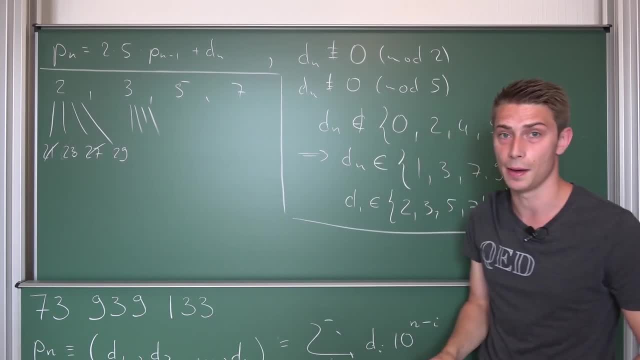 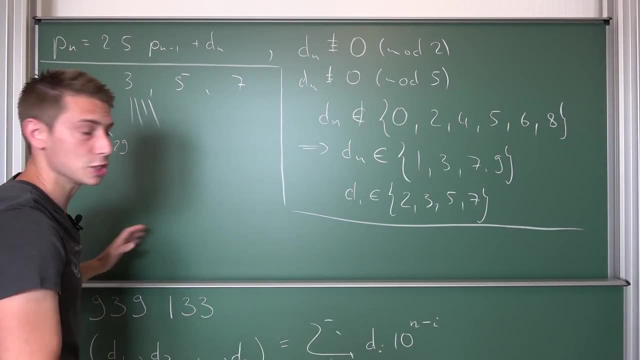 And then for 7.. Then you are going To get a list Of all the 2 digit Right truncatable prime numbers And from this point onwards, We are going To continue This process. Now we are going To take the list. 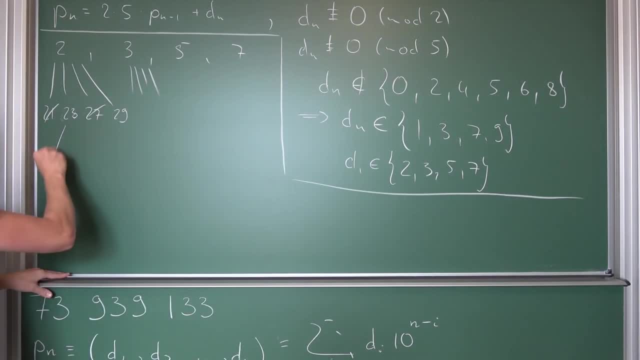 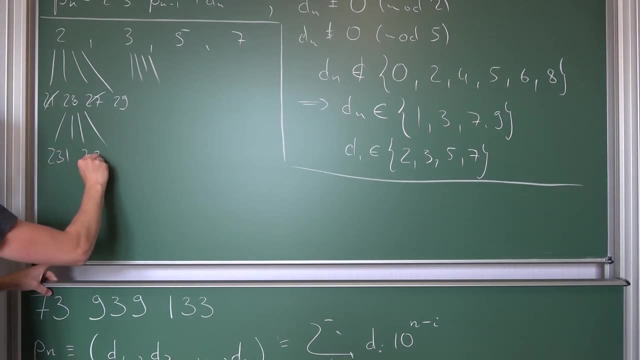 Of all right truncatable 2 digit prime numbers And we are going To append New digits To it. We are going To take 23. And we are going To append New digits To it, Starting with 1.. 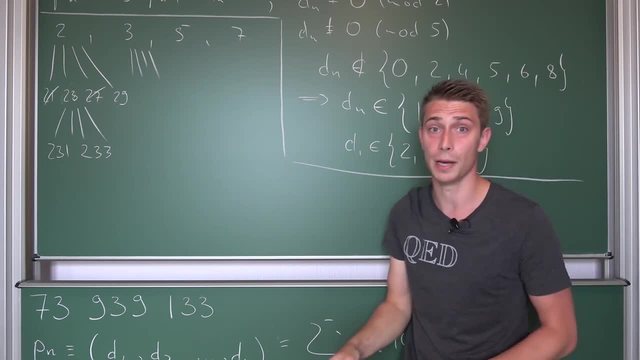 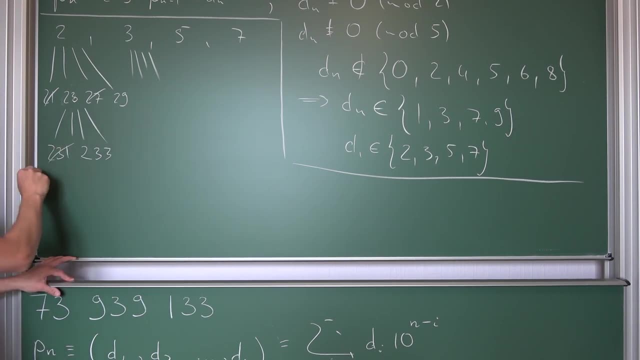 So 231.. We are going To append All the 3 digit Right truncatable Prime numbers. Let the prime number Algorithm Check Run Yet again. So this one Is not Prime Because it's divisible. 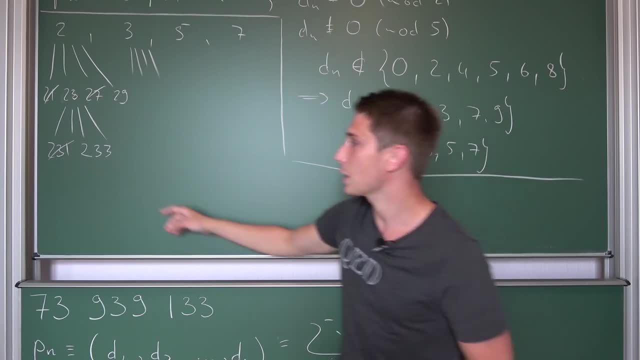 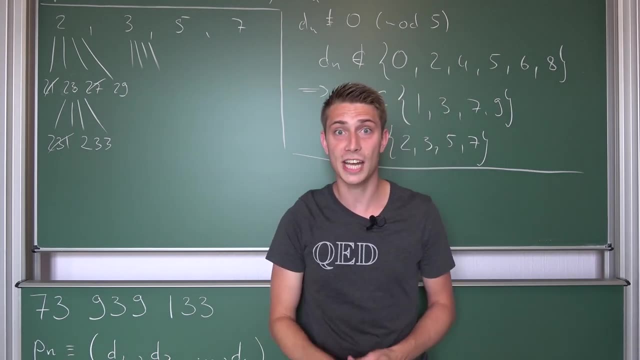 By 3.. But 233.. Should be divisible By nothing, So it's a prime number, And thus We get this, And then we are going To append Those digits Yet again To it, And so on. 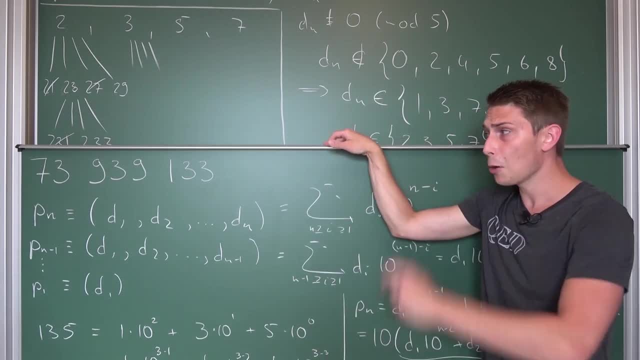 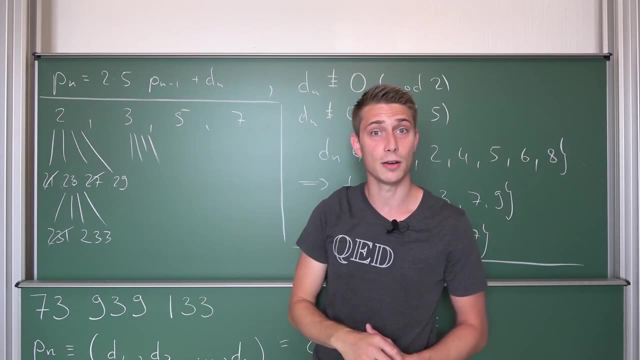 Up until We reach the point Where we have. I hope you understood Everything I said here. I hope this video Was to your liking. If it was, Then make sure To subscribe To the channel And to check out. 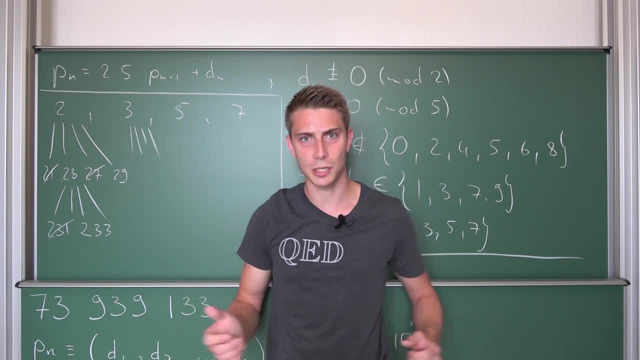 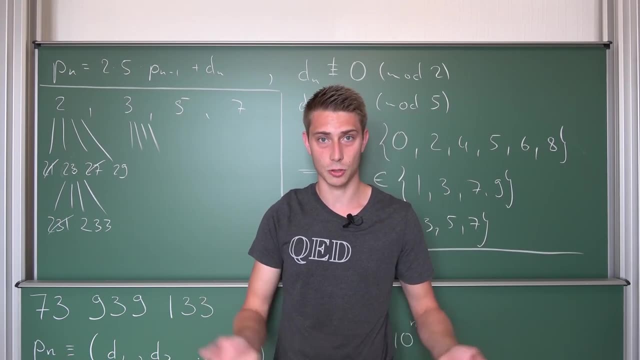 The other videos That come with This very video. And yeah, Thanks again To Matt Park And James Grime For inviting me To this special event. If you have any Big number video That you want to share,